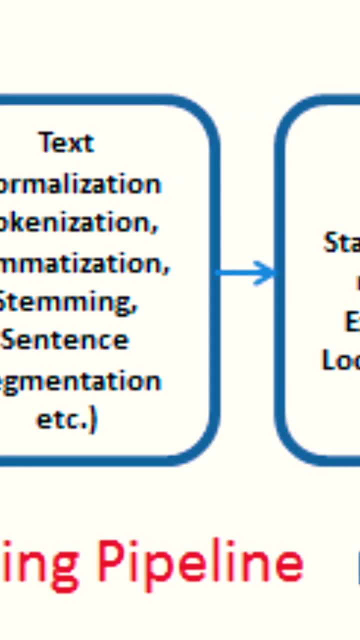 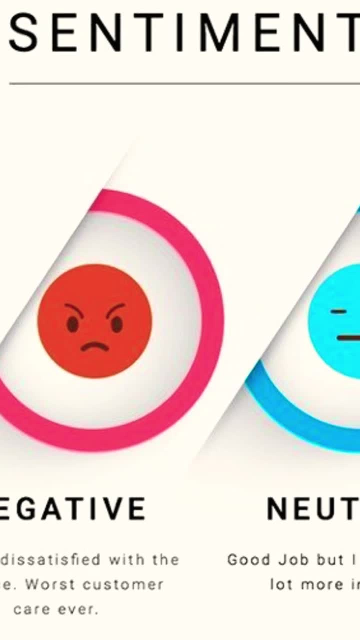 such as removing stopwords and punctuation. Feature extraction involves selecting relevant features from the text, such as keywords or phrases. Finally, sentiment classification involves assigning a sentiment label to the text, such as positive, negative or neutral. 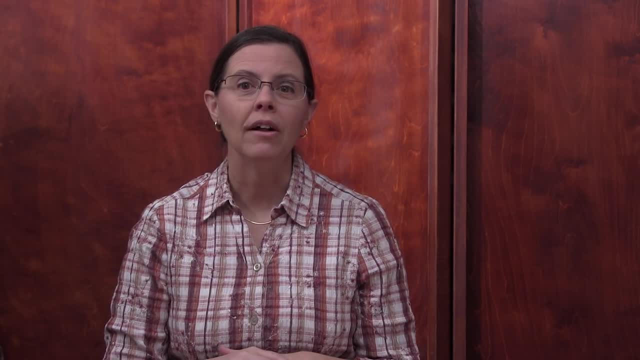 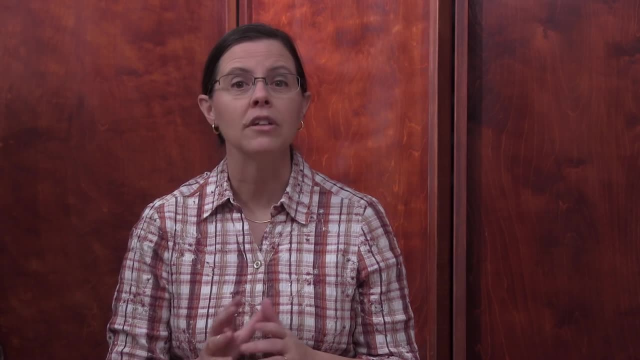 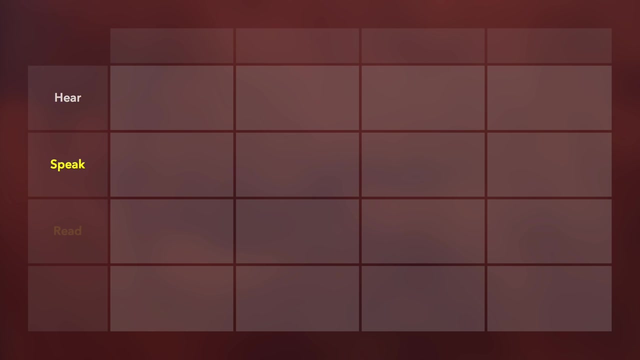 Language arts is simply the art of using language. well, Anything you do to help your child grow in understanding and using language can be considered a component of language arts. When you think about language, you can divide it into four areas: Hearing, speaking, reading. 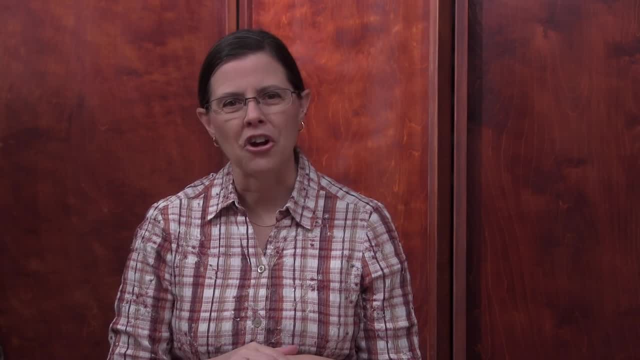 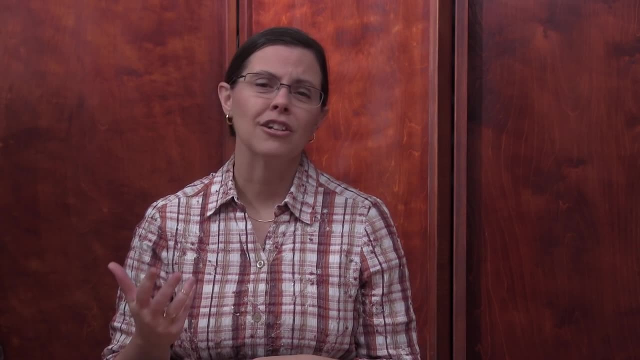 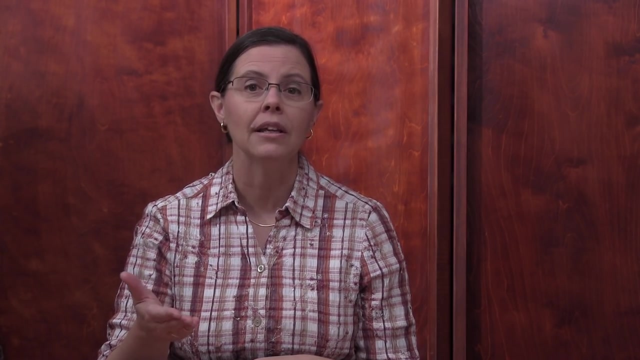 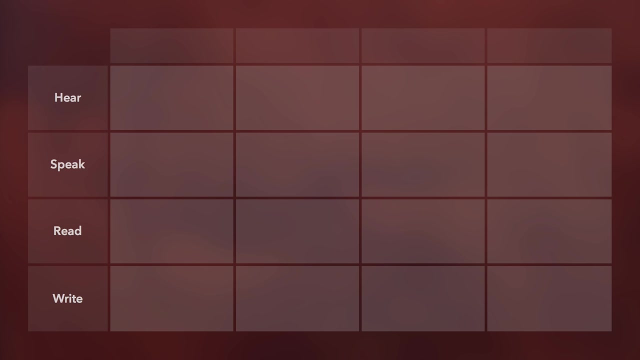 and writing. The main thing to remember about language arts is that learning to use language well is a process, A process that in most cases, occurs quite naturally. Charlotte Mason followed the natural progression of hearing, speaking, reading and writing when she designed how she would approach language arts. Let's look at each of those four areas and see the 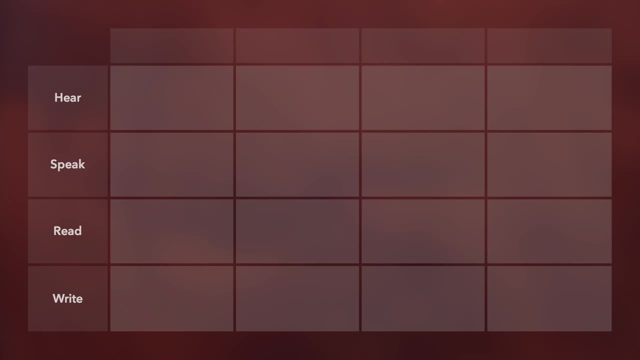